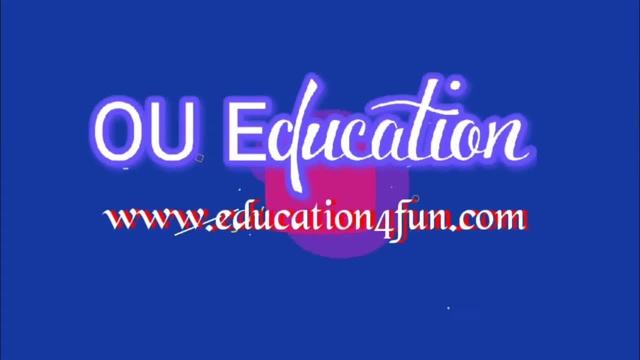 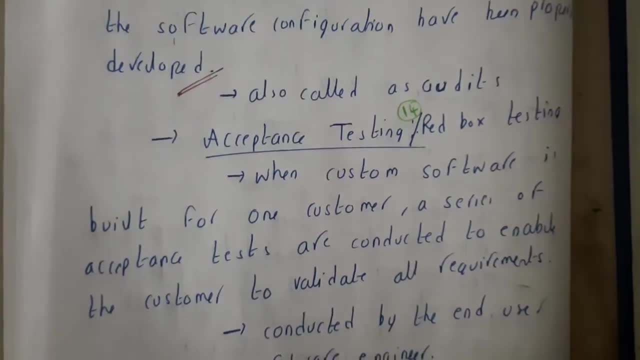 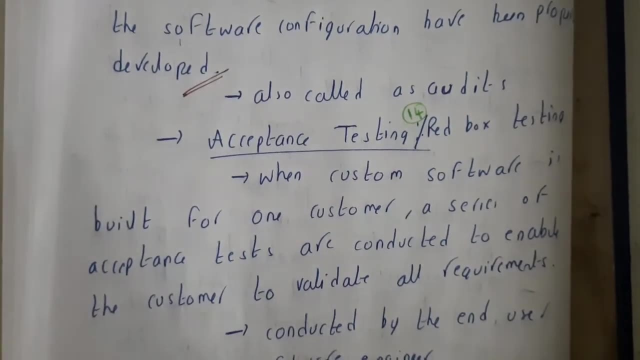 Hello guys, we are back with our next lecture. In this lecture, let us go through acceptance testing, Okay. so basically we have done multiple testings till now, right? Yes, we followed multiple testings like unit integration, okay, And we also gone through evaluation and multiple examples and 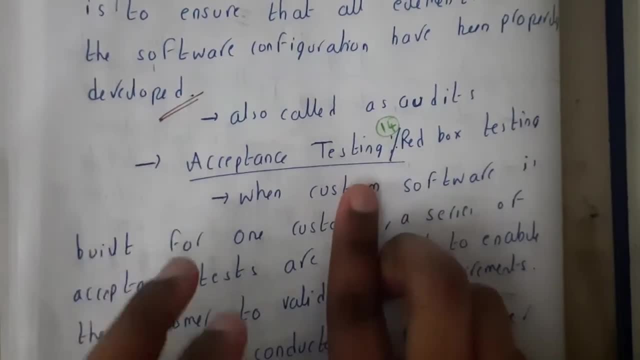 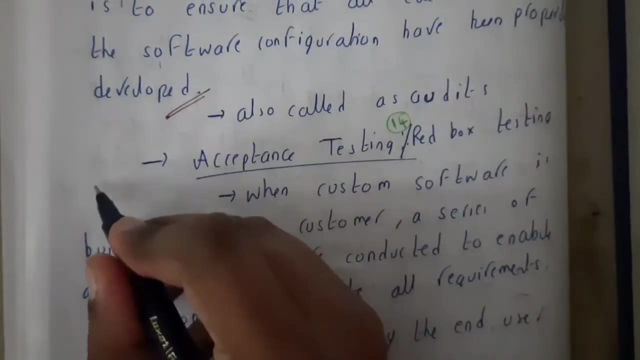 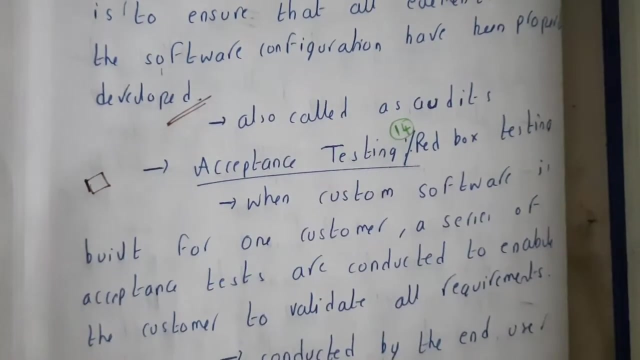 multiple things, right? Yes, so basically acceptance testing is nothing but whether your application is working fine in real world. So basically, when you are testing, so assume you are organizing an event or a fest online, guys. okay, So you took some company and they have told you that you can. 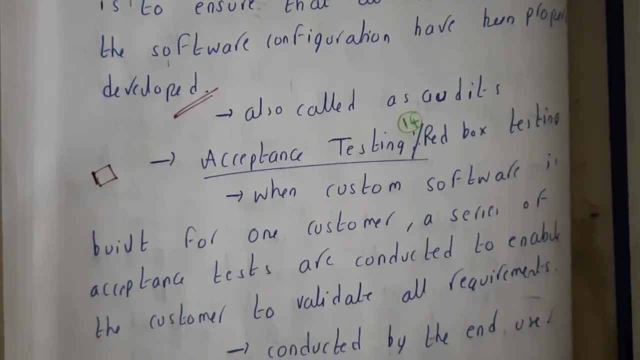 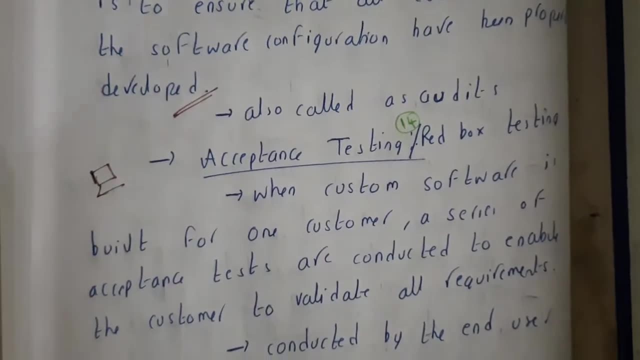 accommodate 10,000 or 1 lakh students. there will be no issues, no technical issues. They told you in that way. So you will be blindly assuming or you will be testing with your faculty, right, So you will be informing your faculty. okay, Let us test this platform. So everyone come on, let us 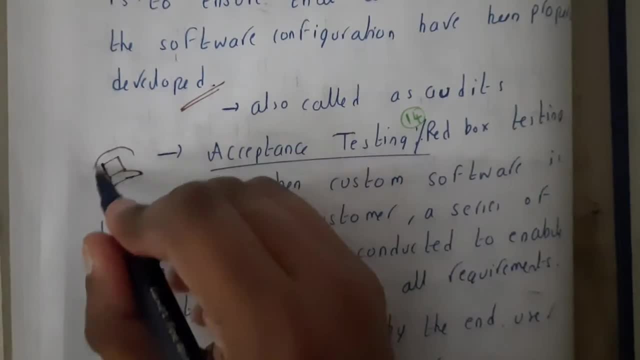 log in and let us try it. So you will be bringing at most 10 or 20 students or 20 people, So you will be 20 faculty only, right? So you will be bringing a minimum number. So at the time of your 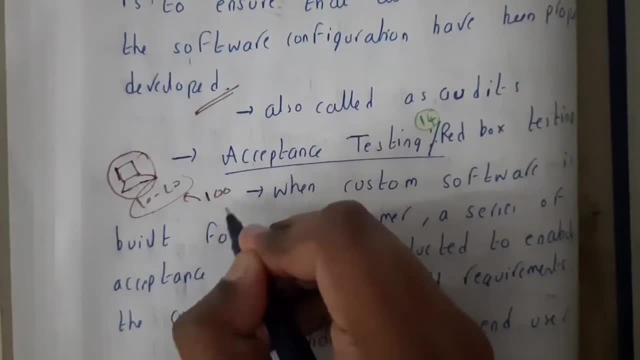 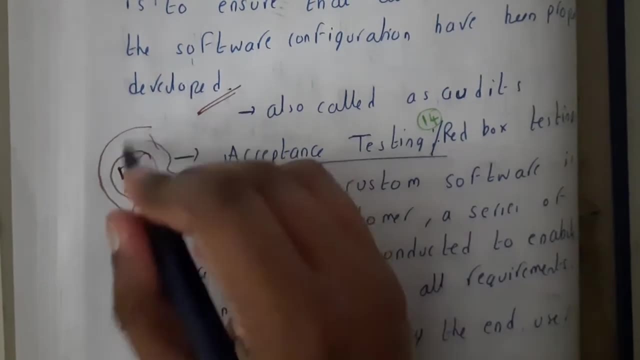 fest, everyone will be logging in, right. So your 1000 or 10,000 students in your college, everyone will be logging in. At that time the server may go down or the server may crash. So these are the commonly seen issues, guys, because even though the software is able to handle, but it is not accepting. 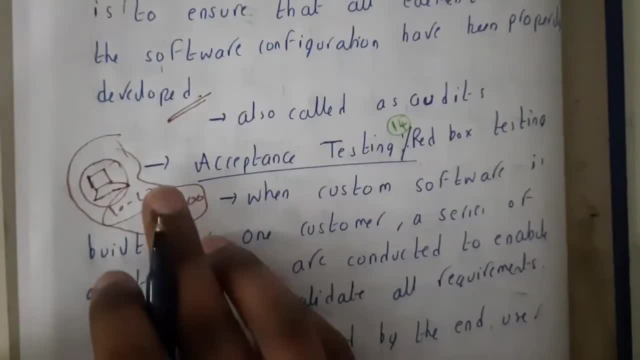 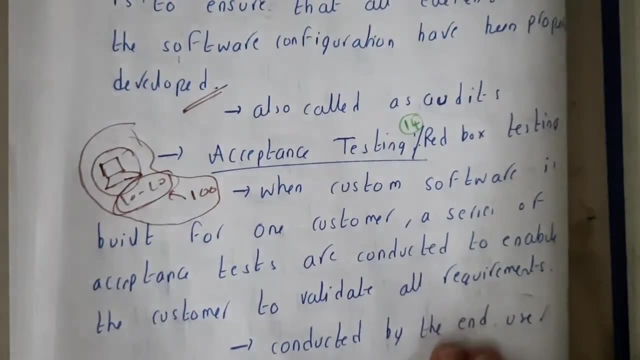 that many users. So that is the issue there. So you can say that their acceptance testing is not done properly by your faculty. So they should check right. So they are checking with 10 to 20 students only Why. They can just inform the students. okay, we are just doing a test run. 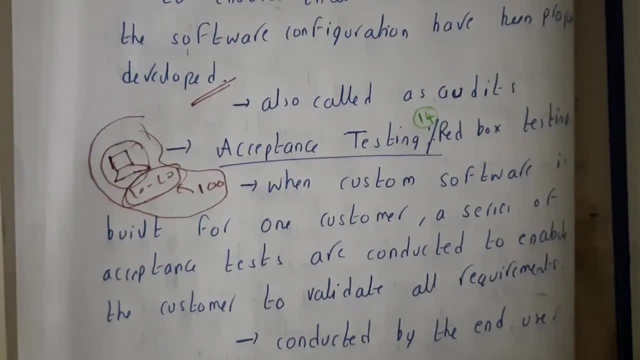 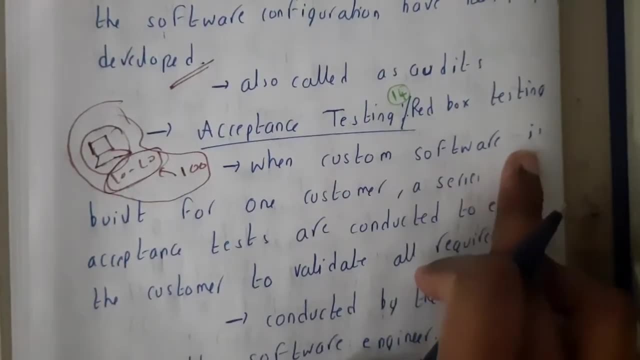 Everyone. please log in and let us test it once. They can ask them right. So they are not doing it properly. So that is nothing but acceptance testing. So it is also called as red box testing. So when custom software is built for one customer, a series of acceptance tests are conducted to. 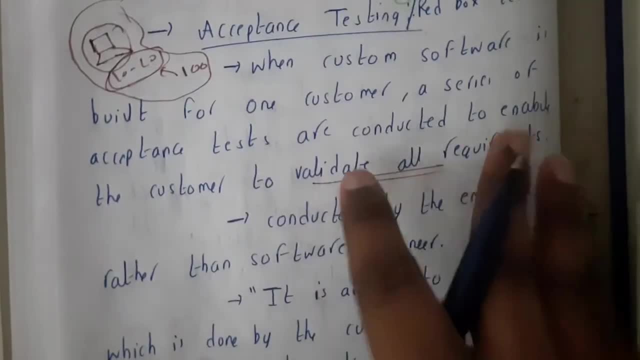 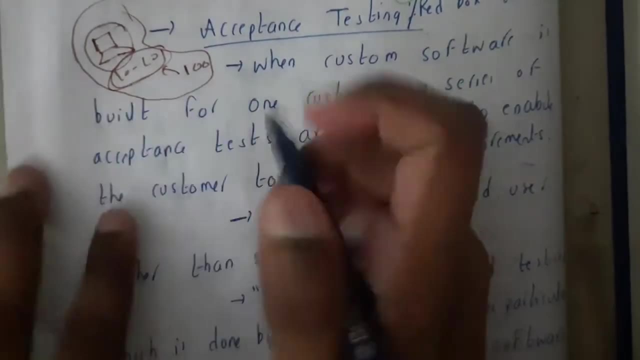 enable the customer to validate his requirements, So he should check according to his requirements, guys. So, basically, when he is requesting the software, he told that he needed to allocate minimum of 10,000 students, But when he is testing, he is testing with 10 or 20 students. That is the main issue, okay, So this is.